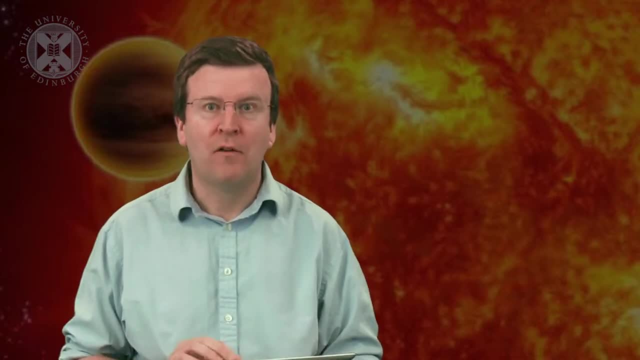 only the suns, because they give light. The planets remain invisible. They are small and dark. There are also numberless Earths circling around their suns. Well, unfortunately, Bruno was burned at the stake in 1600, not just for his astrobiological. 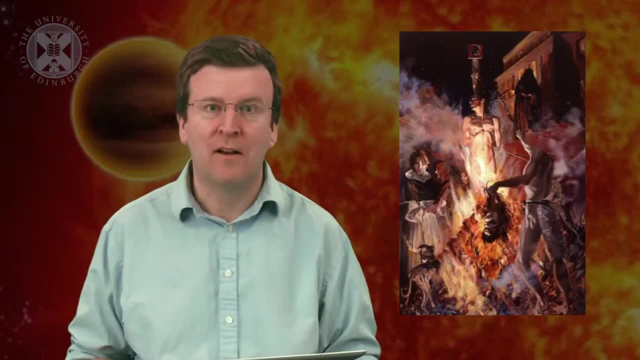 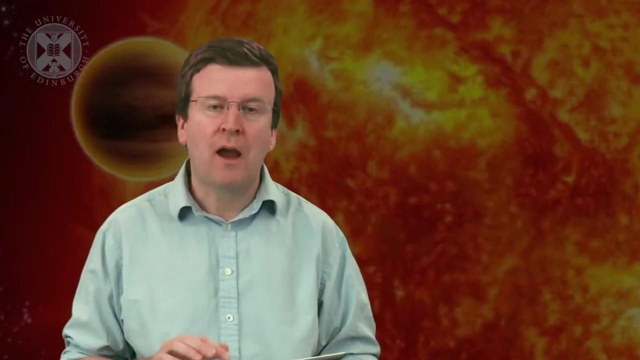 speculations, but also because he did other things that irritated his religious superiors. But nevertheless his speculations about the possibility of planets orbiting other stars, even Earth-like planets, was truly remarkable. The search for planets around other stars really became an empirical science in the 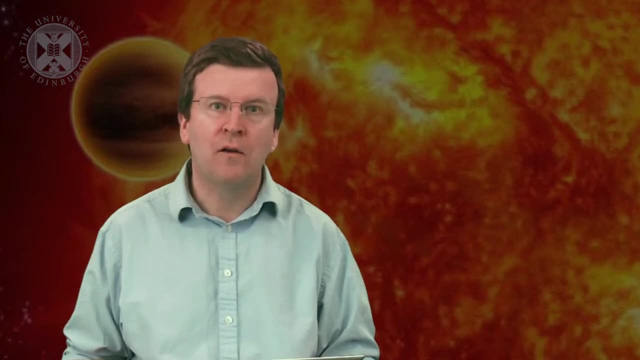 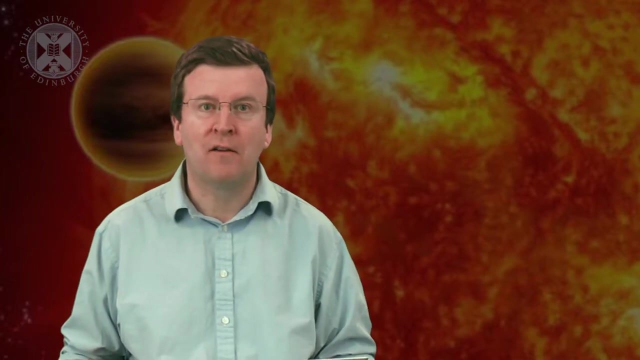 late 20th century. In 1992, two radio astronomers announced the discovery of two planets orbiting a pulsar, a rotating neutron star, And in 1995, Michel Maier and Didier Quelloz of the University of Geneva announced the first definitive detection of an exoplanet. 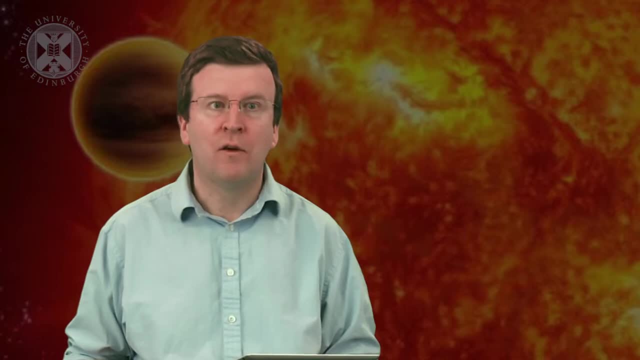 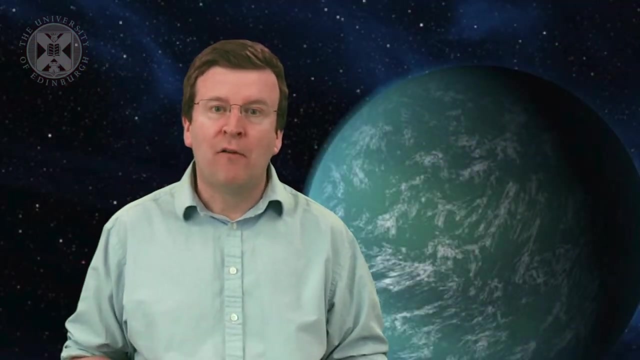 orbiting a main sequence star, a G-type star called 51 Pegasi. These discoveries ushered in the era of the search for extrasolar planets, And now many of these planets are known and continue to be discovered every day, The holy grail for 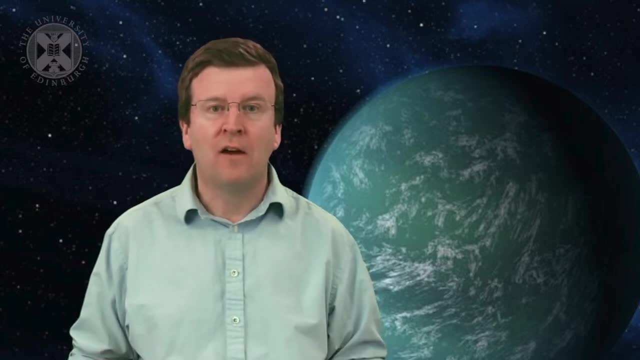 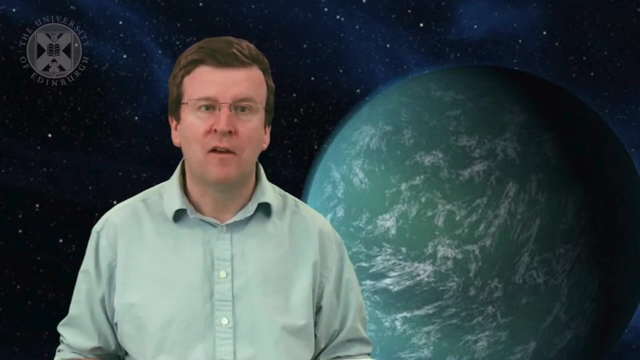 astrobiologists at least, is to try and find a second Earth, A planet identical maybe to Earth in terms of having life and habitable conditions, that may be orbiting a distant star, to be able to detect that planet and study its. 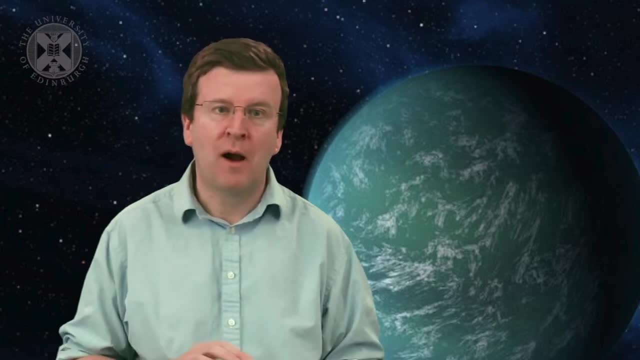 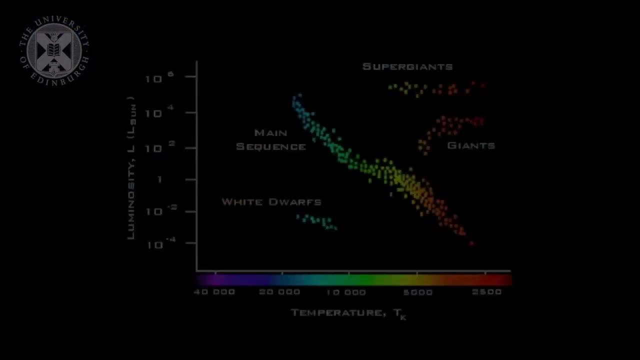 composition, its atmospheric composition and the conditions that it might have to sustain life. The search for planets around other stars in particular is a lot more complex than other stars. has focused on main sequence stars. If we've plot stars according to their luminosity and their temperature, we end up with a 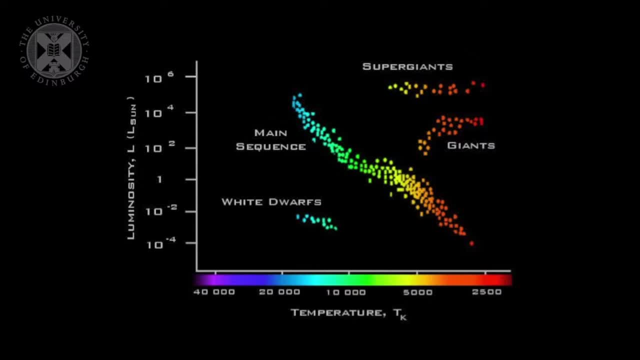 band of stars that you can see in the center of this diagram, the Hertzsprung-Russell diagram, And the majority of planets that we might be looking for are orbiting these so-called main sequence stars, One method that we can use to look for. 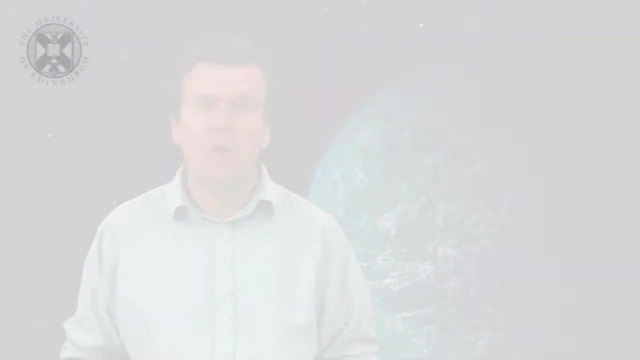 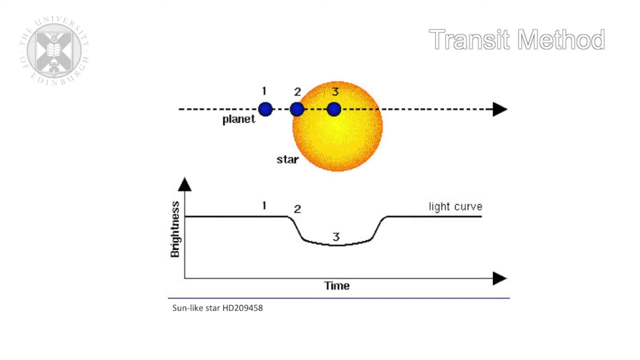 planets around stars is the transit method. When a planet orbits around its star, some of these planets, if they're in the field of light- they're going to be in the field of view of the observer- will pass in front of the star and block. 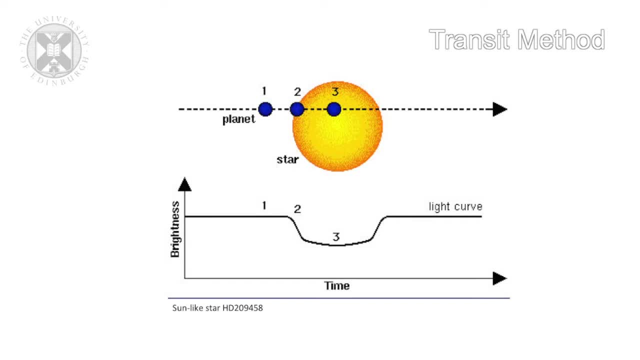 out its light As they block out the light. if you're measuring the light from that star, you'll see a dip in the light given off And this dip can tell you that there's a planet there and something about the nature of the planet orbiting the. 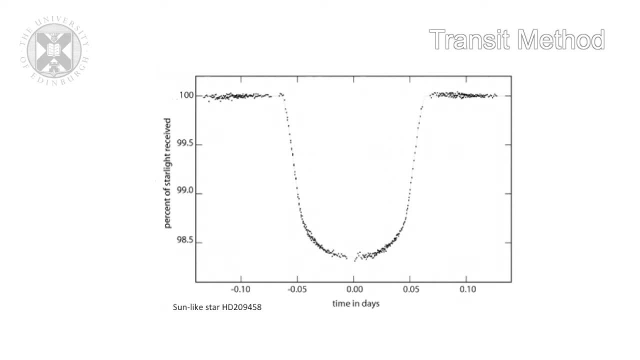 star. This is an example of a light curve from a planet that has transited in front of a star, And you can see very clearly the light of the star continues quite continuously along the top of the graph and then drops when the planet passes. 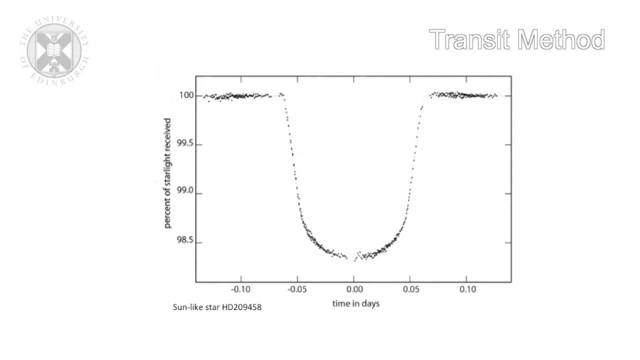 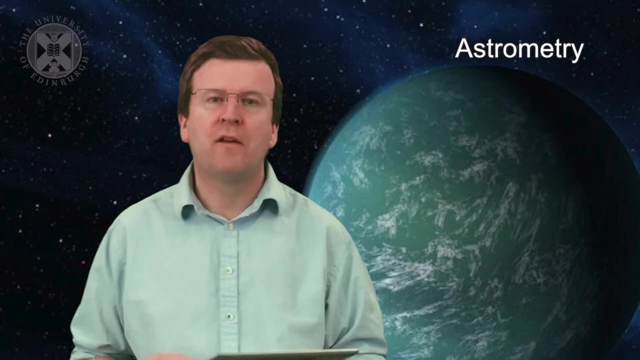 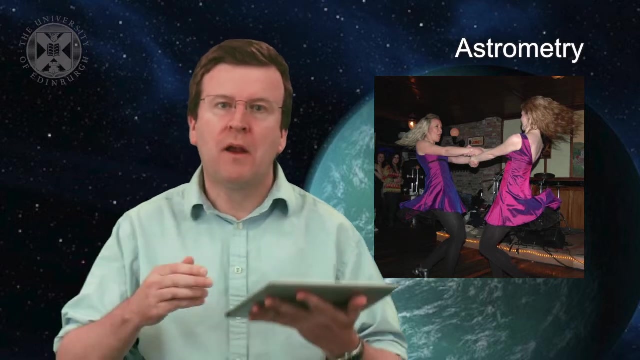 in front of it. This is one method used to search for extra solar planets. Another method to search for planets is called astrometry, And the best way to think about this is to think about two people holding hands and swirling around each other. When two people hold hands and begin to circle around each other, they 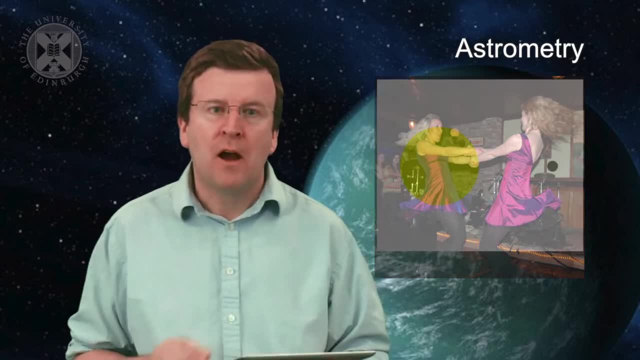 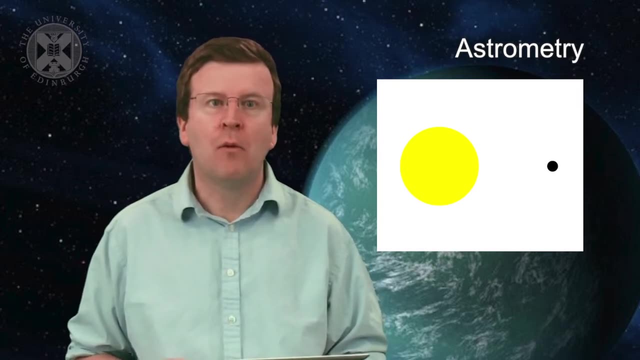 will circle around a common center of mass, And we can use the same sort of method to search for planets around other stars. If a planet is orbiting around a star, they will in fact circle around the common center of mass And the center of 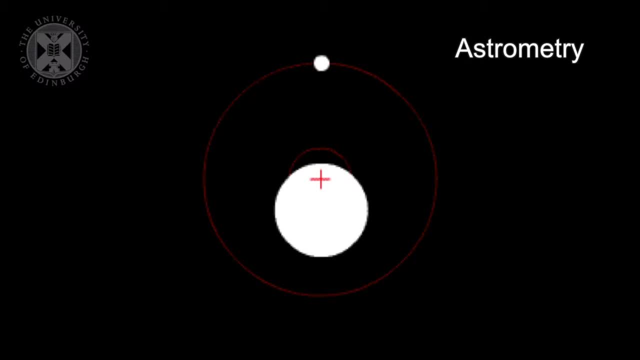 mass will not be exactly in the center of the star because of the mass of the planet. In fact, the star will wobble ever so slightly as the, as the planet and the star revolve around their common center of mass, This wobble in the planet can be. 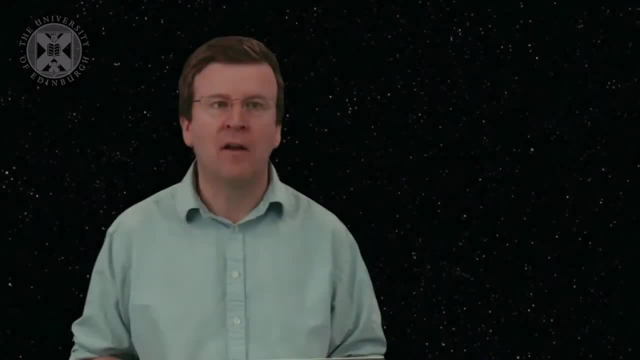 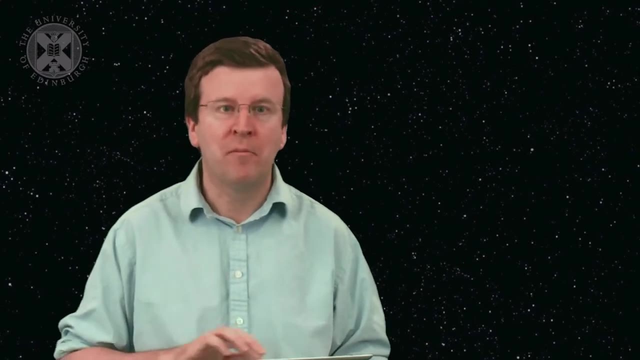 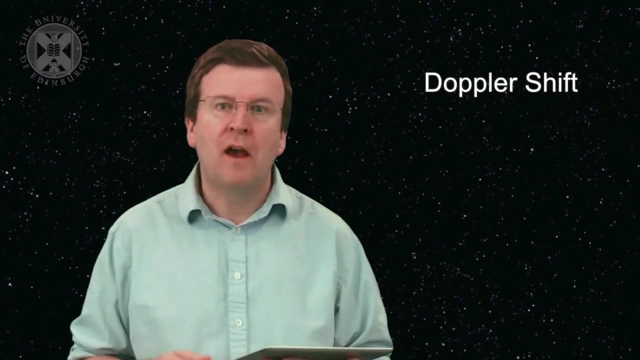 detected and used to infer the presence of a planet. It needs very high sensitivity, but telescopes can be constructed to find planets by the astrometry method. Another method that we can use is called Doppler shift. This rotation of a planet around a star that causes this wobbling will also cause a slight change in the 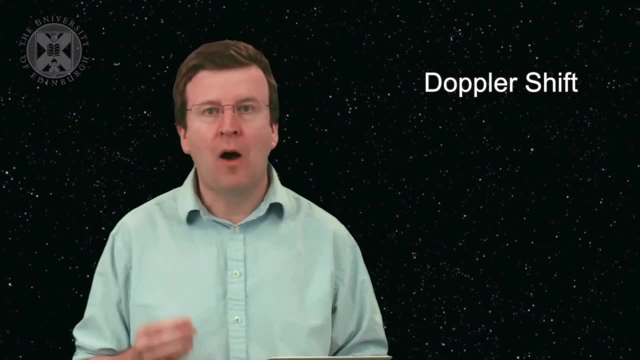 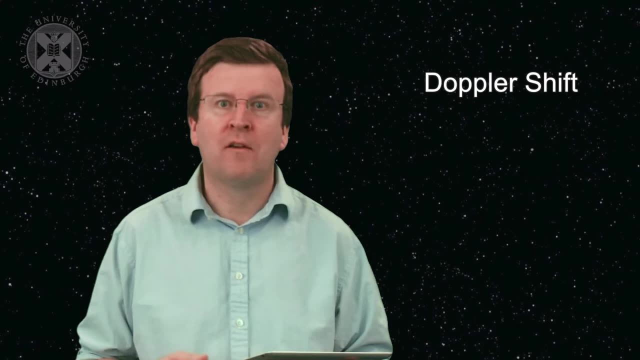 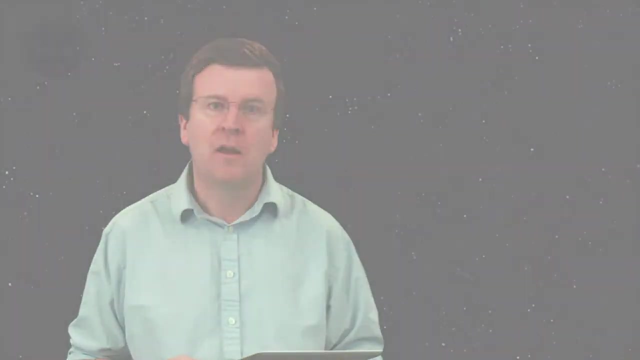 wavelength of light given off by a star. As the star moves away from the observer, the light will be slightly shifted towards the red, And as the star moves towards the observer, the light will be slightly shifted to the blue. This wobbling, caused by the presence of a planet around a star, can therefore be 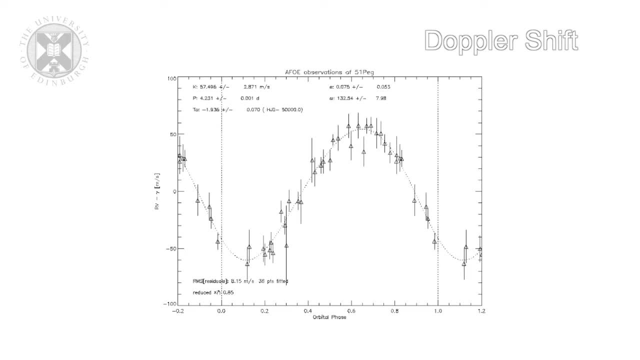 detected by the slight change in the wavelength of the star, And this, this method, called radial velocity or Doppler shift, has been very effective in being used to find extra solar planets, And, by mid 2011,, over 500 stars had been. 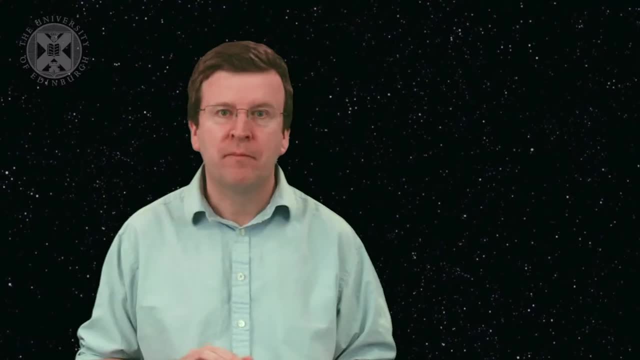 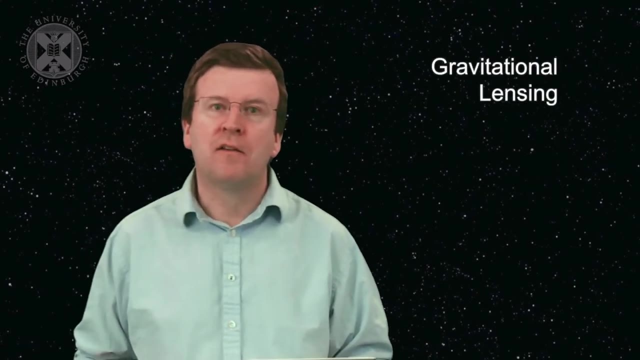 detected using the Doppler shift method. Yet another method that has recently been developed is called gravitational lensing, And the idea here is that a star will distort the light from stars or galaxies Behind it. this is because of the gravitational influence on the light.